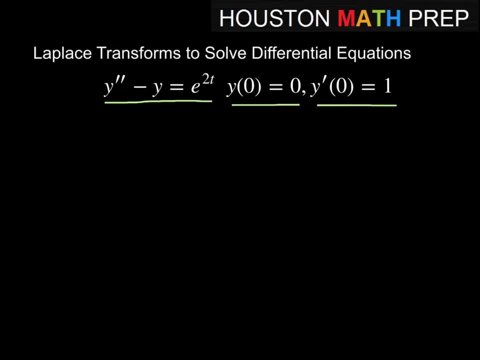 We know what y of 0 is and we know what y prime of 0 is. Okay, so if you recall the Laplace transform of just the function y itself, we called it f of t before. So the Laplace transform of y we said was going to be some other function, capital, Y of s? right? 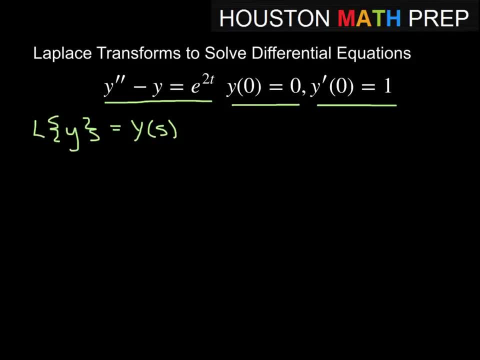 Some new function in terms of s, And when we did the first derivative, the Laplace transform of f prime, here it's y prime. remember that gave us s times this function y of s minus and here it'll be y of 0.. 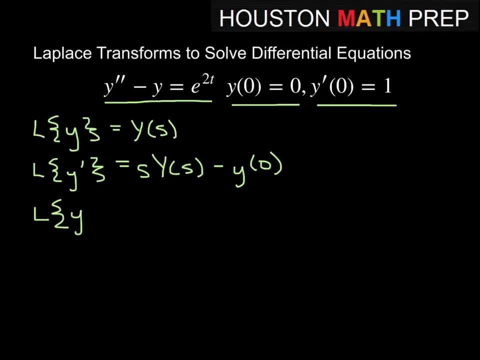 And then the Laplace transform of the second derivative. so y double prime would be s square times y of s minus s. so remember how the pattern goes right: Times y of 0 minus y prime of 0.. So we have all that information and that helps us take care of the left-hand side of the equation. 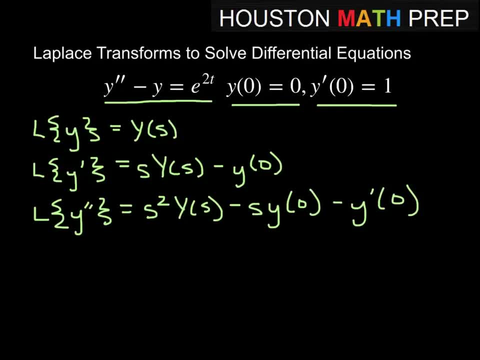 So now the idea is we need to look at this e to the 2t, so we would have to calculate what the Laplace transform of e to the 2t is. So now we either assume at this point that you are starting to memorize Laplace transforms or that you have a table in front of you. 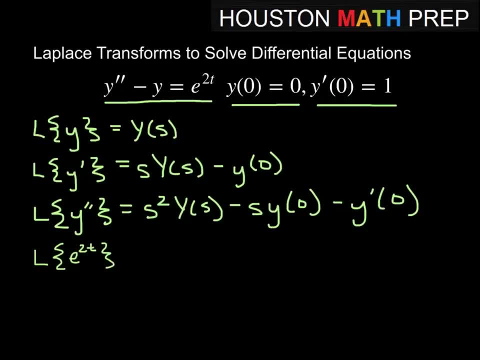 or that you have a table in front of you, because when we get to the end of this problem we're going to have to do the inverse transform and go backwards anyway once we do the algebraic part. So we'll assume that you either are able to look up or have memorized at least some of these basic Laplace transforms. 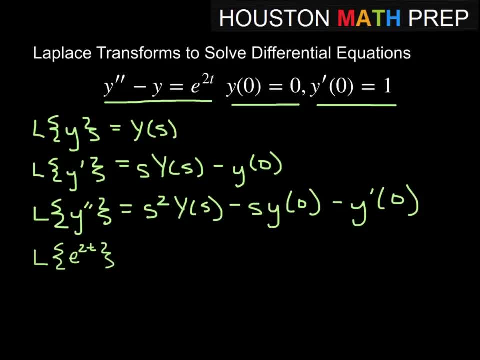 Okay. so if we go ahead and figure out what the Laplace transform of e to the 2t is, it turns out the Laplace transform of e to the 2t is 1 over s squared. Okay, so if we go ahead and figure out what the Laplace transform of e to the 2t is, it turns out the Laplace transform of e to the 2t is 1 over s squared. 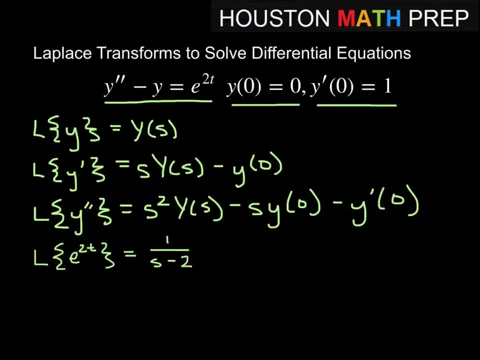 minus 2.. We didn't just pull that out of the air. You can either work that out using the definition or just know that, or look it up on a chart. So our equation here then becomes: so this y double prime, in other words, so we take the Laplace transform of that term, that will give us s. 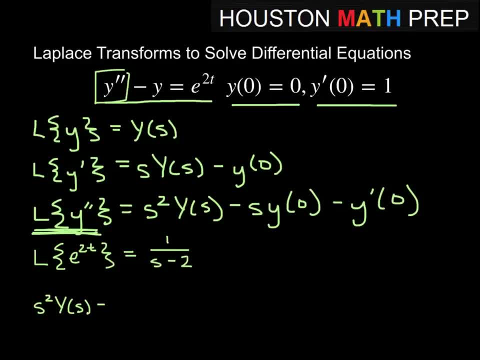 square y of s minus s times y of 0 minus y prime of 0.. So that's our y double prime minus y, right? So this is y double prime minus y and y. the Laplace transform of y is just y of s. 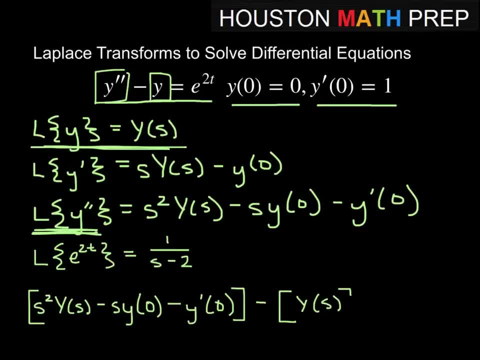 So I'm just sort of putting these in brackets so you can see what each piece is. Equals equal to e to the 2t, and we already said that was going to be 1 over s minus 2.. Okay, so now what we should be able to do is we should start being able to make some substitutions. 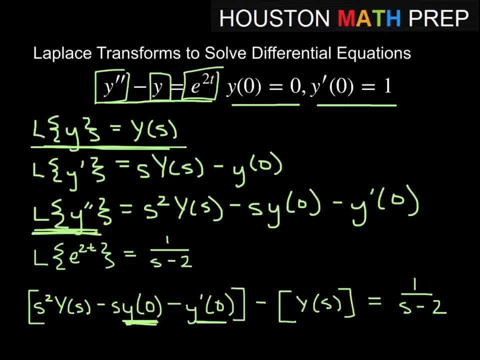 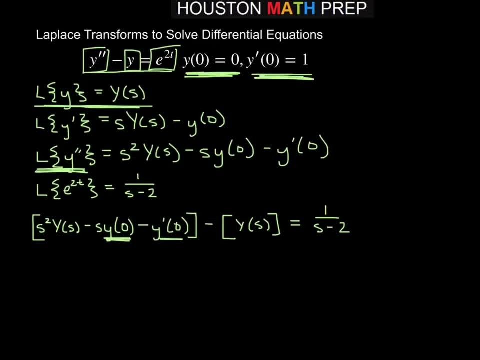 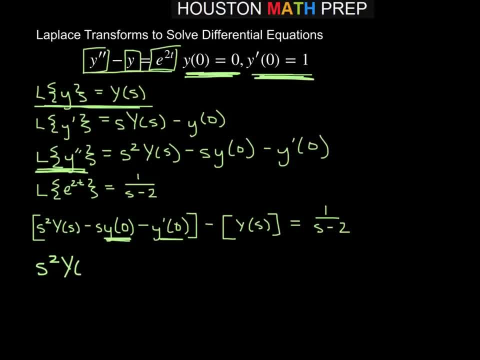 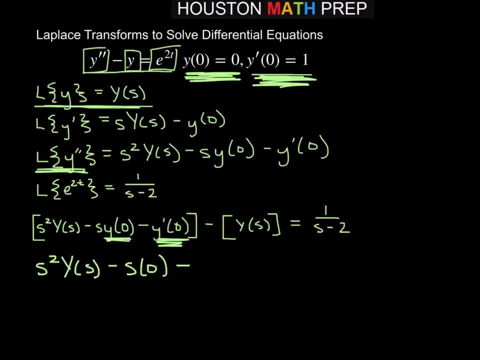 minus y prime of 0, y prime of 0 is 1, so this would be minus 1, and then minus y of s is equal to 1 over s minus 2.. Okay, so now what we want to do is we want to actually. 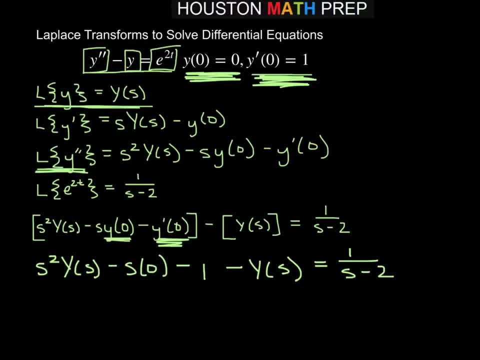 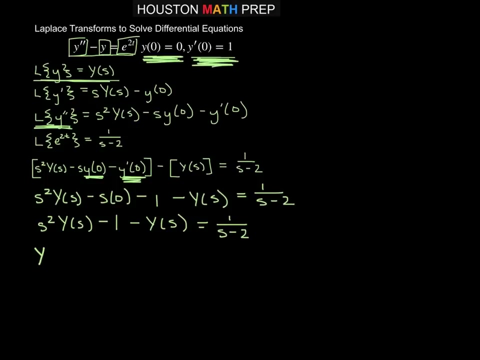 solve for y sub or solve for y of s. so we go ahead and we'll simplify this side here. so we get s square times, y of s minus 1, minus y of s, equal to 1 over s minus 2, and we'll keep going here, and so we get y of s in two separate terms. so 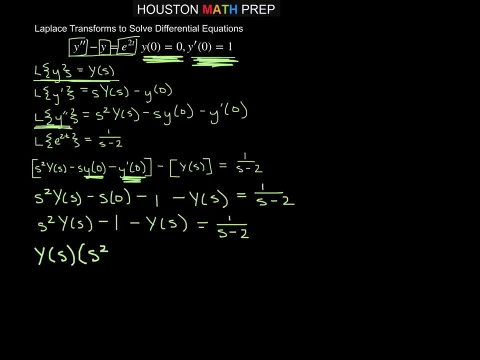 we'll factor it out of the common terms, which would be s square minus 1, and we have this minus 1 by itself. we'll go ahead and add that to both sides, so we'll get 1 plus 1 over s minus 2, and now I'll go ahead and get a common. 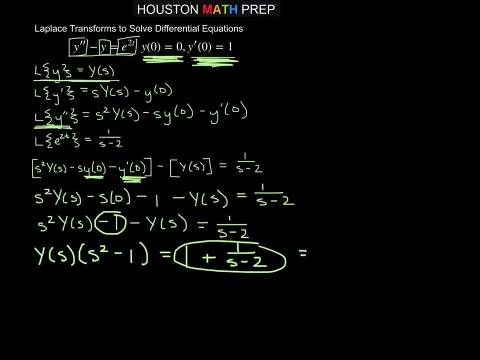 denominator here. so this here would be then: s minus 2 plus 1 over s minus 2. so we can go ahead and say what that is. so y of s times s square minus 1 is equal to s minus 1 over s minus 2, and then we'll just simply divide by this term, that is: 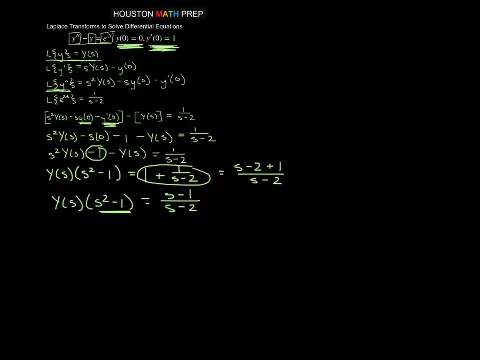 multiplying y of s and we'll get an expression for y of s. so we'll get: y of s is equal to s minus 1 over s minus 2 times s square minus 1, and we can simplify here if we notice that that quadratic expression will factor. so we'll get s minus 2 times s. 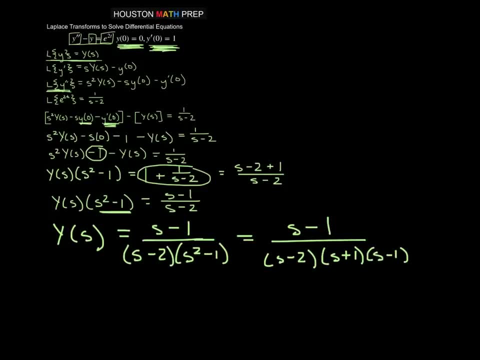 plus 1 times s minus 1, and we'll reduce both of those to 1, so we'll get y of s is then equal to 1 over s minus 2 times s plus 1. so it's at this point in time that we want to use partial fractions to continue working with this and simplify. 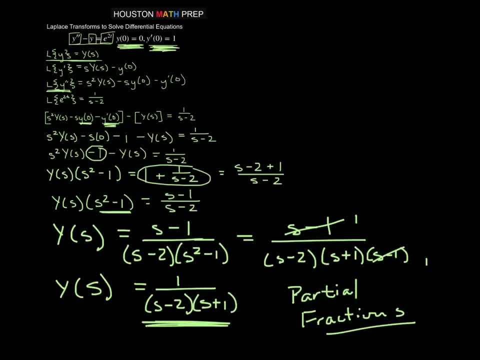 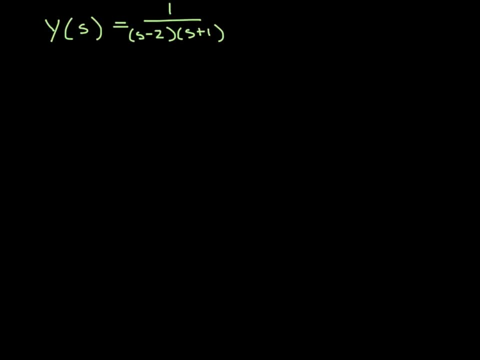 So we would need to get a partial fraction decomposition for y of s. Okay, so if we write down what we have so far, we're going to get partial fractions here. so in other words, we have one over s minus 2 over s plus 1. we're going to assume everybody is okay with partial. 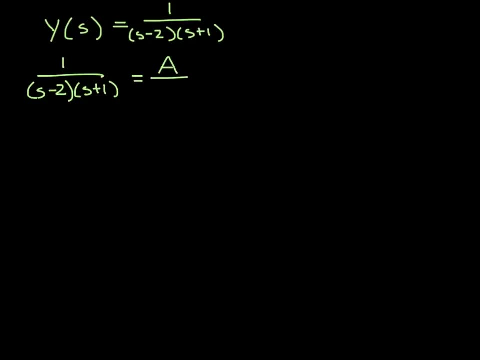 fractions. so we have linear factors here. so we'll have a over s minus 2 plus b over s plus 1, and remember we'll multiply in whatever missing to get a common denominator. so we would end up with 1 equal to a times s plus 1 is missing. 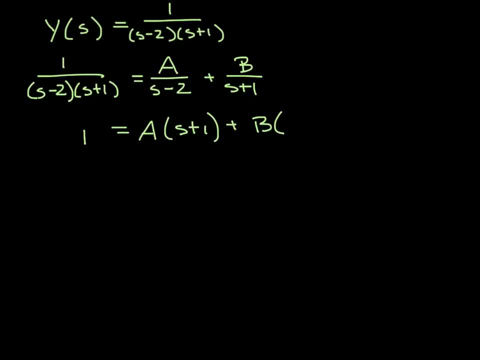 underneath a plus b times s minus 2 is what's missing underneath b. So we could go ahead and set each factor equal to 0, and so if we let x- sorry, if we let s- equal to negative 1,, then that 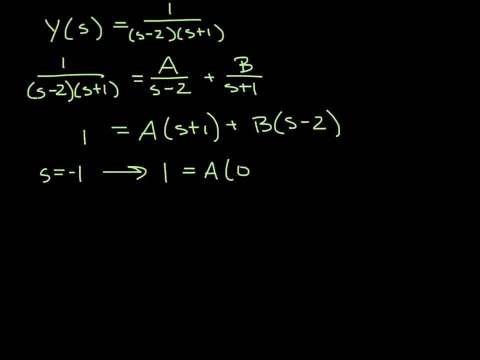 will give us 1 is equal to a times 0 plus b times negative 3, and if we let s equal to 2,, then that will give us 1 is equal to a times 3 plus b times 0.. Okay, so from those expressions there we get. 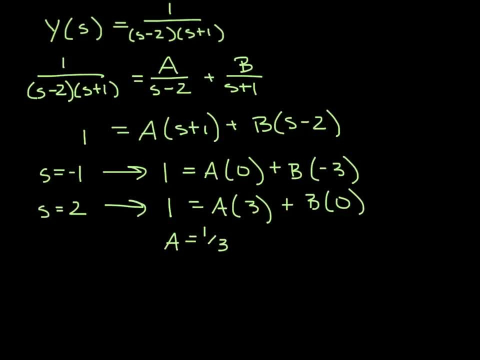 that a is equal to 1 third And b is equal to negative 1 third. if we solve both of those equations for a and b, Okay. so if we go ahead and use this information then and we plug it in here, then that tells us y of s is going to equal 1 third over s minus 2 minus 1 third. 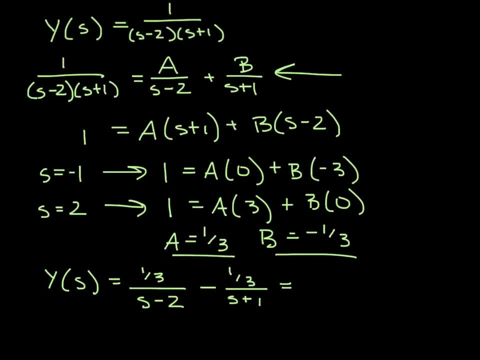 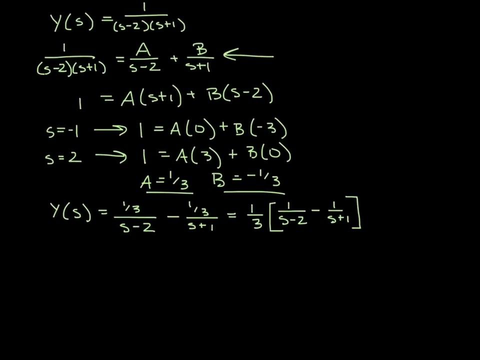 s plus 1.. Another way you could say this is that this is actually 1, third times, I guess: 1 over s minus 2 minus 1 over s plus 1.. Might be another way to say that. Okay, so now it has come to the point where we do the inverse transform. So you either want to know those or get out your chart for that. 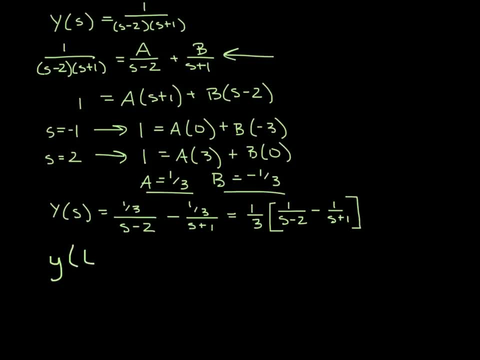 Whatever our y of t is, our original solution for y- that's what we solve for- is actually going to be the inverse, Laplace transform of whatever y of s is. So we're going backwards. now We're doing the inverse transform. Usually, when we take the transform of y, we get capital Y of s. If we take the inverse transform of y of s, we get the original function y of t. 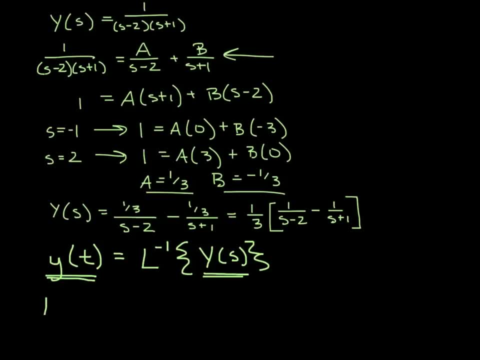 Okay, so in other words, we get the inverse Laplace transform of y of s. So in other words, the inverse transform of y of s would be the inverse transform of our expression here: 1, third times the quantity 1 over s minus 2 minus 1 over s plus 1.. 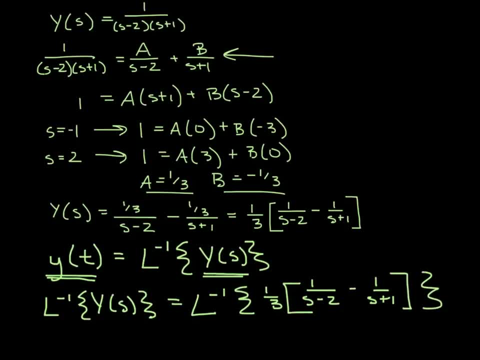 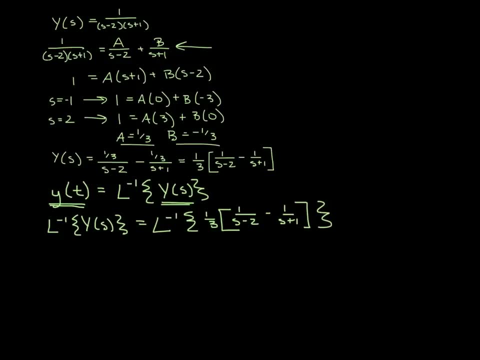 So we're taking the inverse transform of that. So we have that constant multiple of 1 third which we can go over here. So we're going to go ahead and bump out according to our transform rules there. So in other words, y of t would equal 1 third times the inverse transform of the stuff here, right? 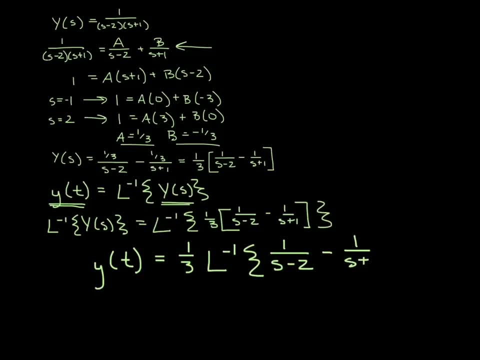 1 over s minus 2 minus 1 over s plus 1.. Okay, if you look in your formula chart or if you know these, then these are both going to be dealing with exponentials here. So we have 1.. 1 third and then the first one here, because it's 1 over s minus 2, that's actually e to the 2t according to your chart probably. 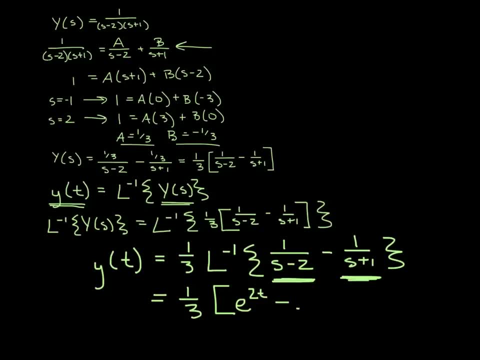 And then we have minus, and because this is plus 1, we use the opposite sign, so that's actually e to the minus t there. Okay, and so that is our solution. y of t equals 1 third, or you could distribute the 1 third if you would prefer there. 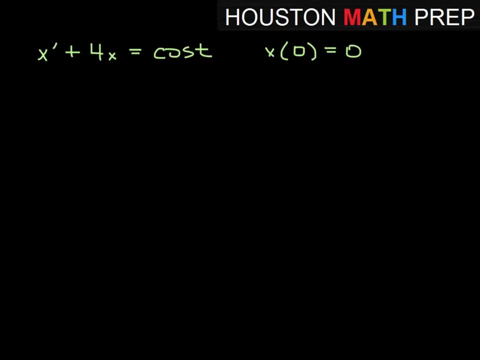 All right, and we'll look at 1.. Here we'll do a first order equation. So here instead of y primes we have x primes, So x is a function of t here. So we have the first derivative of x plus 4x equals cosine t and we have our initial condition: x of 0, equal to 0.. 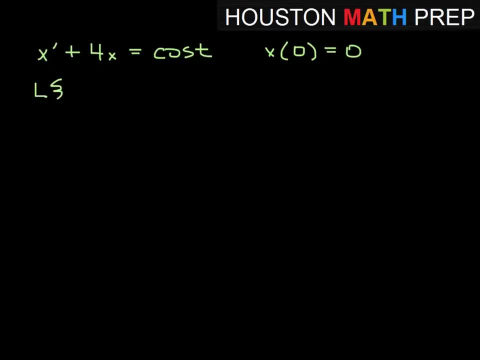 So we'll look at our Laplace transform. So our Laplace transform of x or x of t is just going to be big X of s And our Laplace Laplace transform of x prime or x prime of t, according to our formula, is going to be s times x of s minus x of 0.. 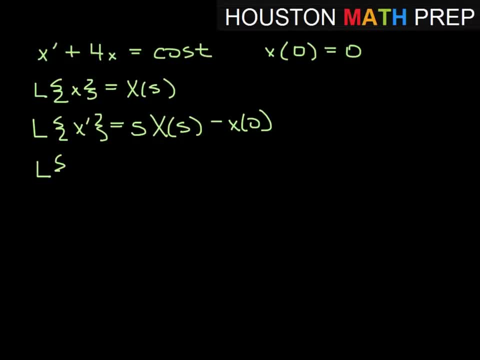 And Laplace transform for the right side. we'll need the Laplace transform of cosine of t, So we can work that out using the integral definition or start to memorize some patterns if you've already done that. We've already worked with these several times and so we'll get that. the Laplace transform of cosine t is going to be s over s squared plus 1.. 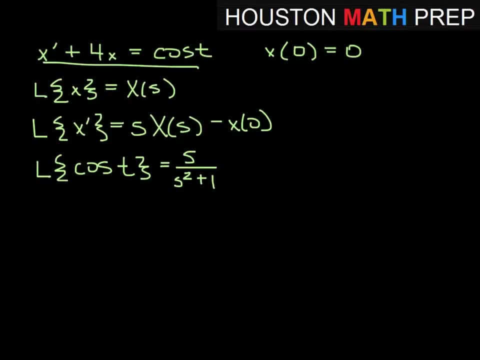 All right, and so now we'll put in all of our Laplace transforms for each term. So Laplace transform for x prime is x times x of s minus x of 0, plus 4x, so plus 4x of s. 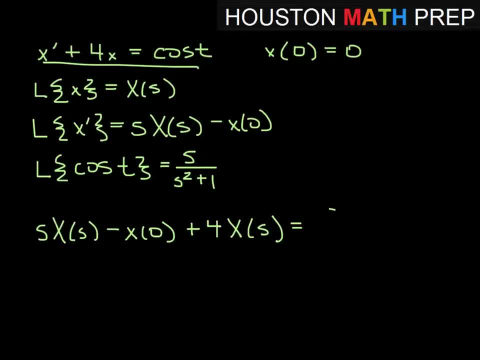 That's the left side, equal to the Laplace transform of cosine t, which is s over s squared plus 1.. And now if x of 0 equals 0, then that means this term here is 0.. So that will give us, on the left-hand side, x of s times the quantity s. 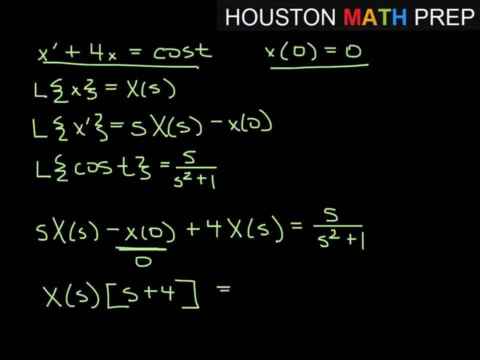 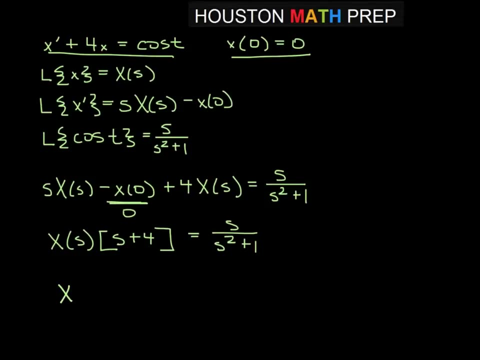 Plus 4, equal to still s over s squared plus 1 on the right-hand side. Okay, so if we solve then for x of s and divide by s plus 4, then that will give us x of s is equal to s over s plus 4 times s squared plus 1.. 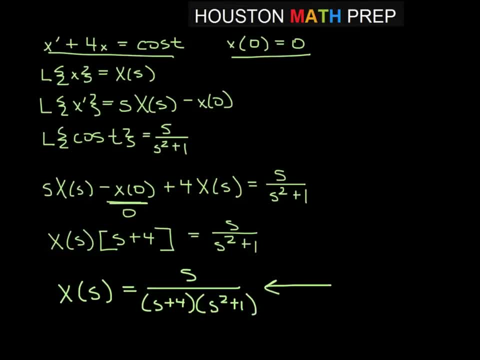 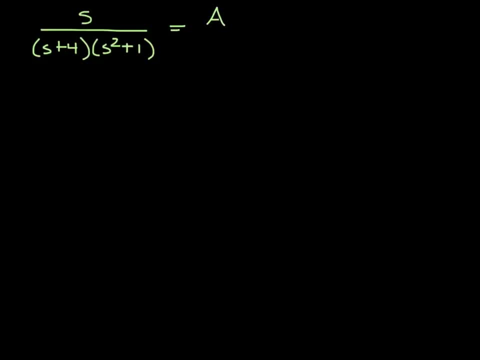 So for this expression here now we will do the partial fraction decomposition for that. Okay, so if we're doing partial fractions for this, so we have a linear term, so that would be a over s plus 4.. The second term is a quadratic factor that's not reducible. 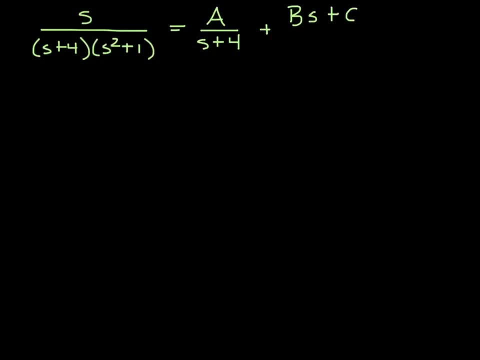 So here we will set up bs plus c over s squared plus 1.. So we need a linear factor, A linear expression. So we need a linear expression, So we need a linear idea over the quadratic factor. So getting common denominator, then that will be s equal to a times s squared plus 1. 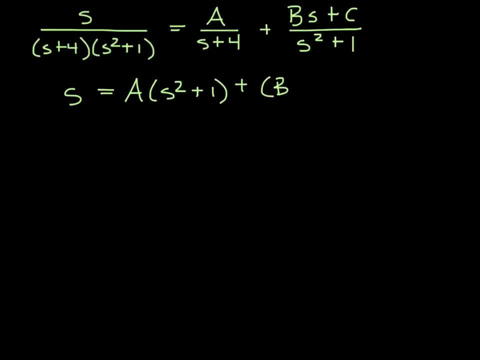 plus bs plus c times s plus 4.. So we could at least use negative 4 to make this factor equal to 0. So let's do that. So if s is equal to negative 4, then that will give negative 4 is equal to. 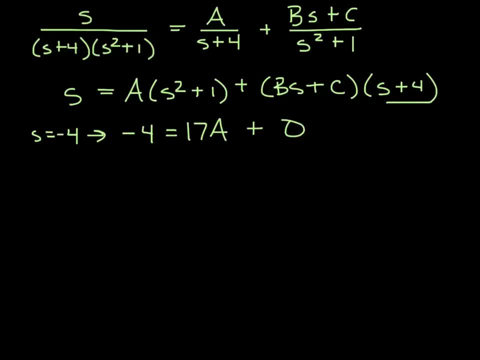 17a plus, and all of this would become nothing over there. So a would equal negative 4 over 17. And then we can't make this factor 0, so we'd have to compare coefficients. so we'll distribute on both sides. 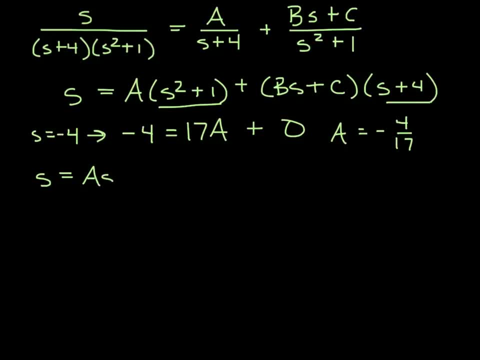 So s equal to as squared plus a plus bs, squared plus 4bs- There's a joke in there somewhere- plus cs plus 4c, All right, and so comparing coefficients. So if you think about, remember what we do here. 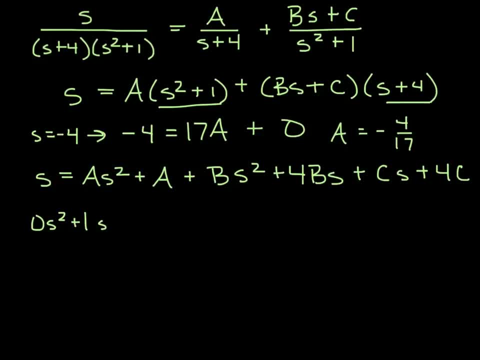 So we have 0s squared plus 1s plus 0 on the left-hand side is really what we have Over here. we have a plus bs squared. if we combine the like terms And then for the b terms we have or the s terms we have, 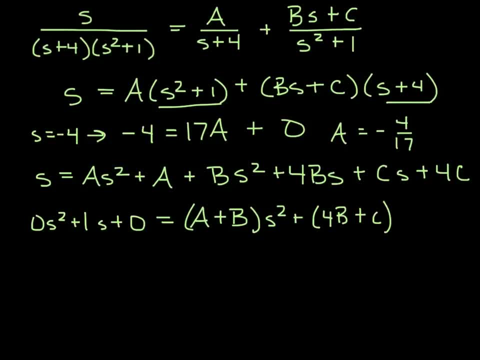 4b plus cs terms, and then we have plus and we have a plus 4c for the constant terms. So we just compare coefficients. giving us a plus b is 0,. giving us 4b plus c is equal to 1, and a plus 4c is equal to 0, if we compare coefficients, 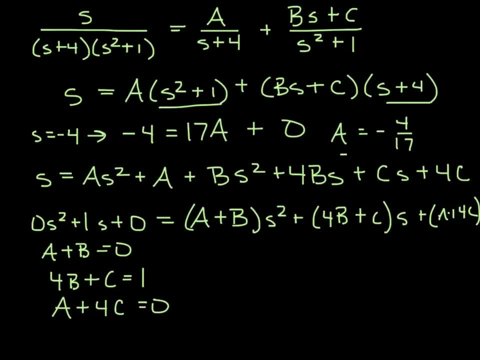 Okay, so now from here it looks like, since we already know that we have a plus b, we know a is negative 4 17ths. If we use this one, we will get that b is equal to positive 4 over 17,. 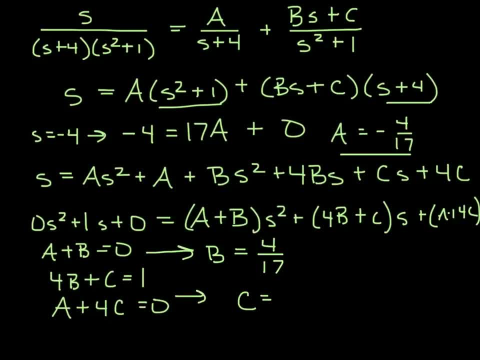 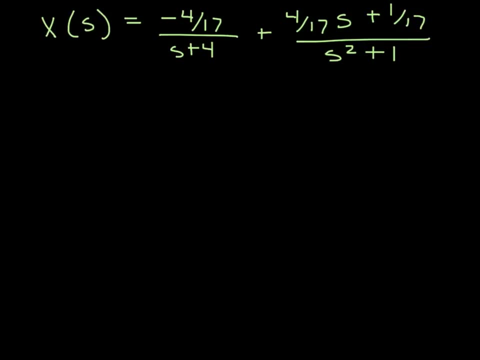 and then, if we use either one of these, I think we should get that c is equal to 1 over 17.. So we'll take that, that and that and put it in here. Okay, and so now this gives us our partial fraction decomposition. 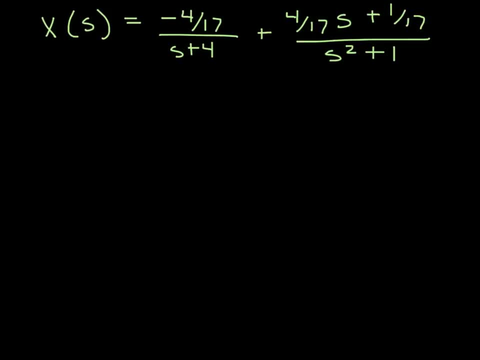 So x of s is equal to a over s plus 4 plus bs plus c over s squared plus 1.. And so now we just simply need to rearrange these in terms of Laplace transforms so that we get our s's or our k's, or however we have them memorized. 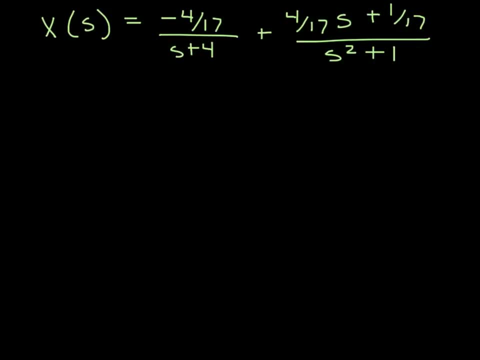 or in our chart, if we're going off of a chart for the inverse Laplace transform. So I'm going to go ahead and make some adjustments here and I am going to go ahead and pull out the negative 4 over 17.. So I'm going to make this negative 4. 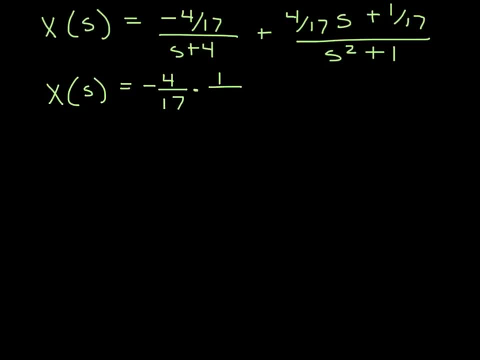 over 17 times 1 over s plus, 4 plus, and then I'm actually going to split this second fraction, So I'm going to make this 4 over 17 times s over s squared plus 1, and then I'm going to write plus 1 over 17 times 1 over s squared plus 1.. 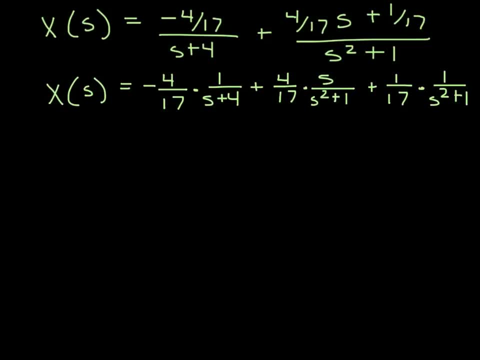 So now I'm going to go ahead and pull out the negative: 4 over 17 times 1 over s squared plus 1.. Now these should all fit nicely if we're familiar with or have a chart in front of us for, particular inverse Laplace transforms. 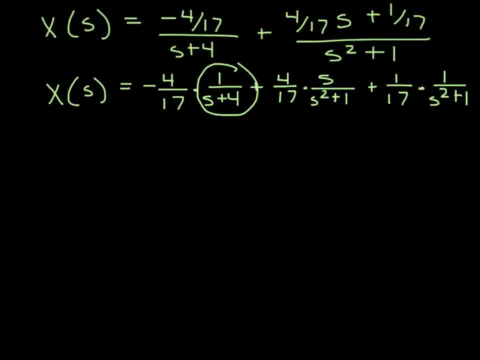 So going off this 1 over s plus 4 term, and when we take the inverse Laplace, transform of everything. so this will give us x, or x of t if you prefer to write. So this would be negative 4 over 17,. 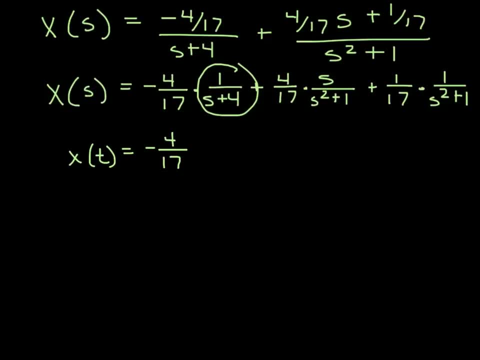 and that 1 over s plus 4, we have that linear factor with a plus 4, so that's going to give us e to the remember. it's opposite what we see. so minus 4t here And then for the next term. so I'm going to get plus 4 17ths. 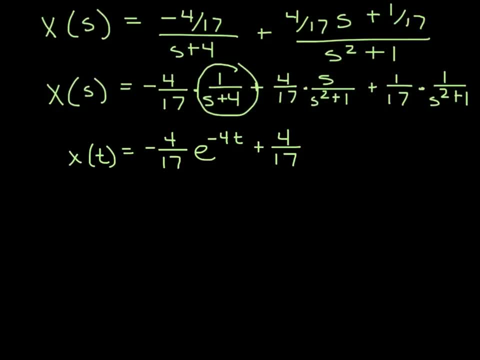 and s over s squared plus 1,. that might be looking pretty familiar to you, because that appeared early in the problem. That was actually exactly the Laplace transform for cosine of t, And then we also have plus 1, 17th, and now 1 over s squared plus 1,. 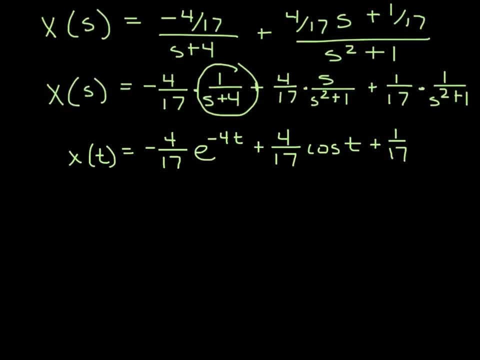 a little bit different but very similar. that is actually the Laplace transform for sine of t. So here, just either using our knowledge of Laplace transform or going off of a chart and working backwards, we took the inverse Laplace transforms of all three of these terms. 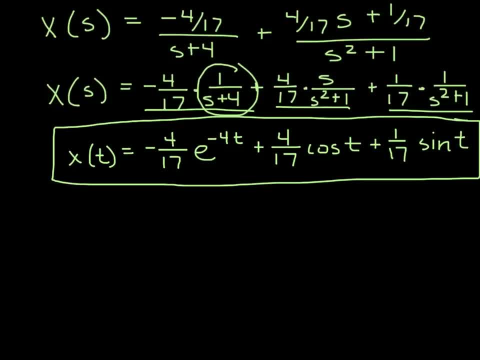 and arrived back at our solution. x of t equals negative 4 17ths e to the minus 4t, 4 17ths cosine t and 1 17ths sine t. Okay so these are two examples. We did a first order equation and a second order equation.